have Traceroute. So on Windows platforms you have Traceroute, The RT at the end is short for route. And on Linux Unix systems you have Traceroute. So on Windows platforms you have Traceroute- The RT at the end is short for route. And on Linux Unix systems you have Traceroute. So on. 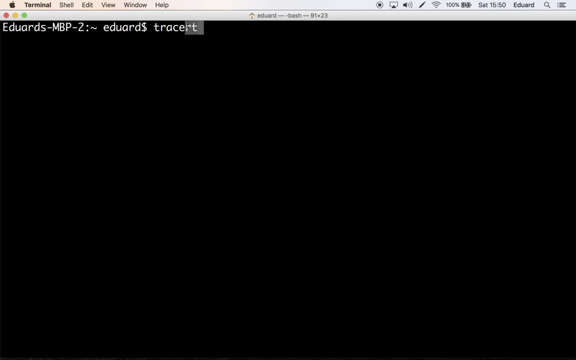 If you're on Windows, make sure you follow the instructions shown in this video, but replace Traceroute with TracerT. In our case we're in the Mac terminal, but if you're on Windows you need to open command prompt and that's located in start programs accessories, and then you should be able to see. 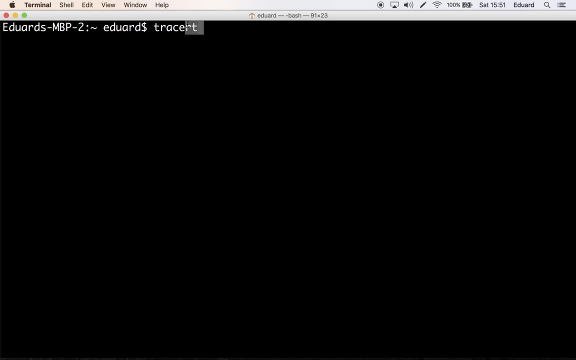 command prompt. Sorry for digressing. I wanted to make you aware of this distinction in case you're running Windows Back to Traceroute. This is a very important tool and it's being used by network engineers all over the world to determine the source of network issues. 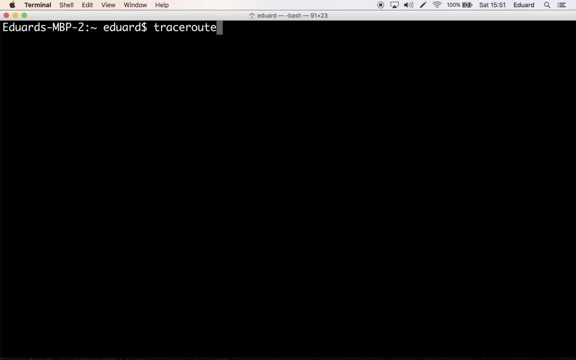 when these emerge, If they have issues with the server or any other device, Traceroute can help them out, and can help you out too, if you decide to do network troubleshooting yourself- in telling you where the issue is Right. so, without further ado, let's run the command and let's say we want to. 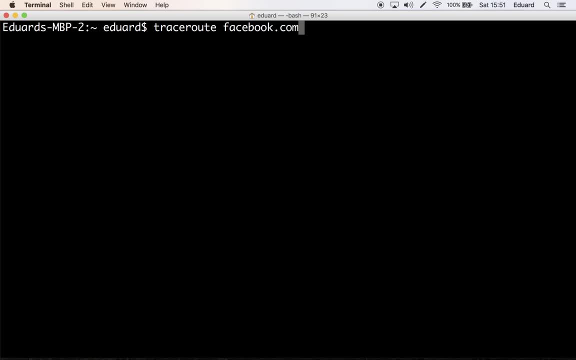 traceroutefacebookcom- press enter. Each line in the output gives specific details of interaction with each router encountered. So it showed details as the name of the hub or the router, its IP address and besides these you'll see three run-trip times. 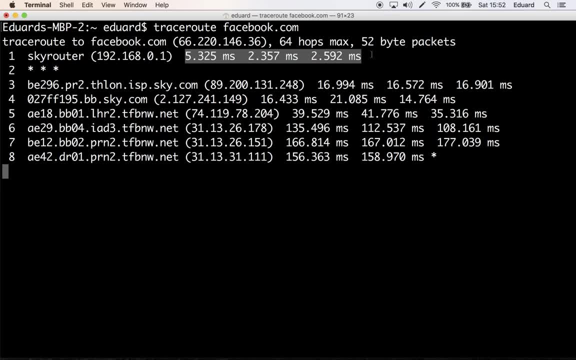 times for that particular router or hub. Traceroute fires three packets when you run it and this output will show three roundtrip values, one for each packet. Virtually Traceroute works by sending packets, by increasing the TTL or the time to leave value. 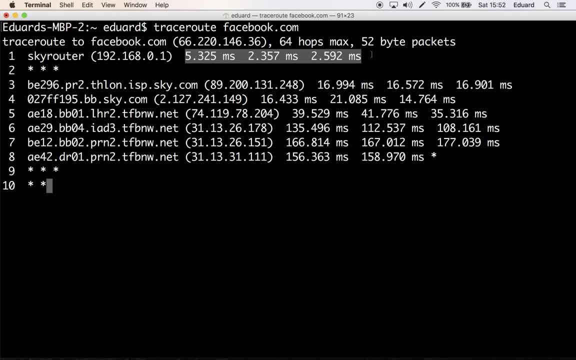 one by one. So initially it starts at one and the maximum, as shown here, is 64.. So TTL is the number of hops a packet can take before being dropped. As the whole value is incremented, Traceroute is able to build a list. 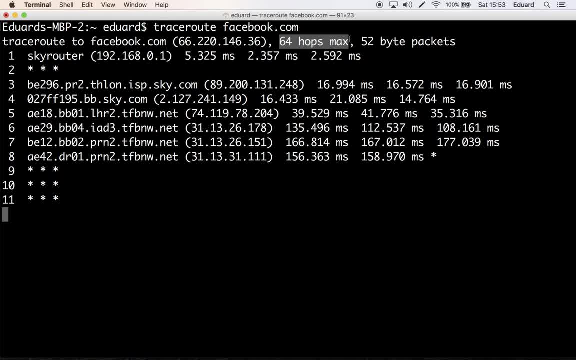 quite a comprehensive list of routers between you, the user and the host destination. In my case, the first router Traceroute Encounters is my Sky router in the first line and then it goes to a PR router and that should be a Provider router. 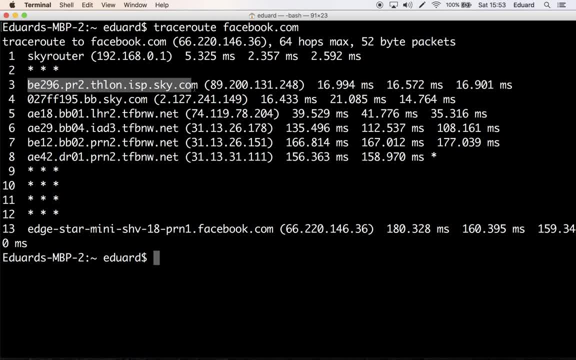 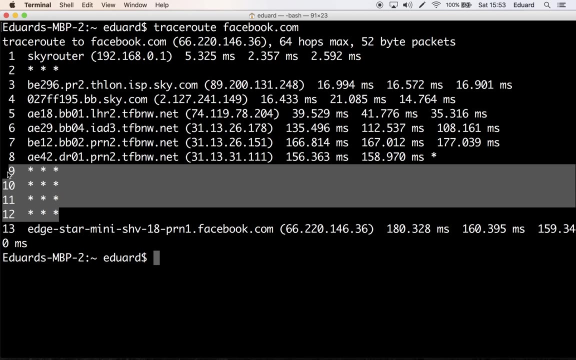 and this is, in all probability, a Sky SuperCore router. Then the route is traced all the way, all the way down to facebookcom, Right. so sometimes you'll see an asterisk in the output, As you can see here. rather than a value, This is simply a timeout that tells you that that field could not be fetched, And reasons for this timeout can be anything from reverse DNS lookup failure to packets not reaching the target router or packets getting lost on their way back, or even the TTL value not being enough. 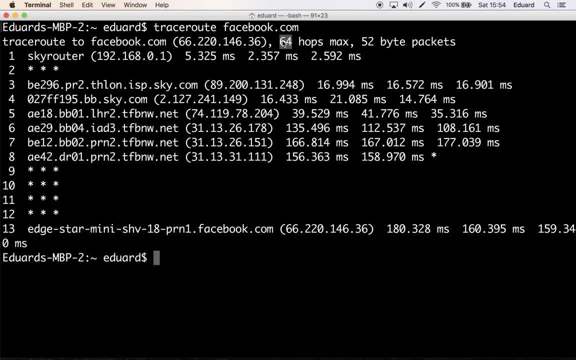 As you can see, here we have a 64, which means when it reaches 65, that packet gets discarded. Anyway, regardless of the case, this utility provides an asterisk in the output. So, as you can see, using traceroute, you can visualize the path your traffic takes between your computer and a specific destination. You could use an IP address as an argument or a domain name. 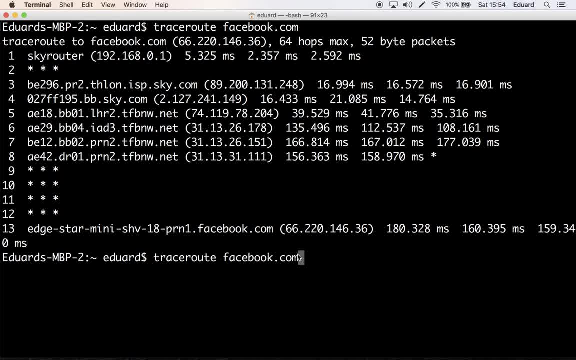 Like we have here. this is the domain name facebookcom. But if you do decide to use a domain name but don't want to see all these domain names listed in the output, but just let's say their IP address, you could simply use a dash n option and it will clear the domain name from the output. 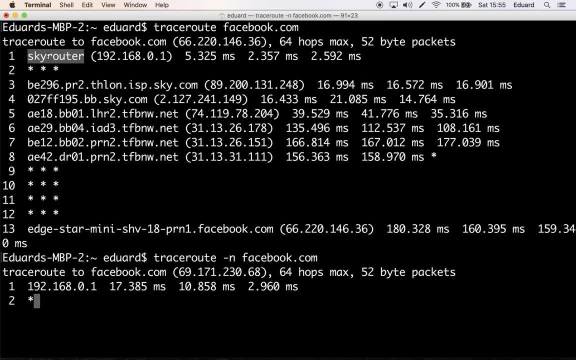 It no longer lists the domain name- in my case skyrouter- but it lists its IP address, as you can see here in the output. Right, let me just cancel this command. So there are other options that could be used with traceroute, but I'll show you the most important ones. 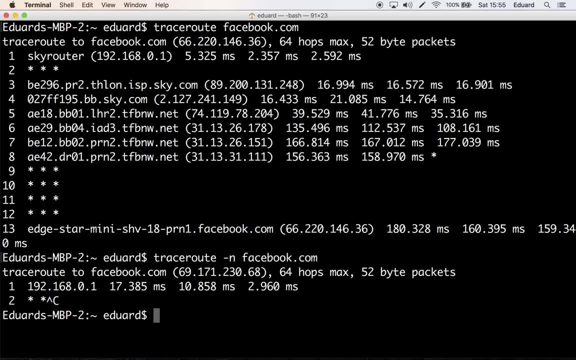 As mentioned before, by default traceroute fires three queries per router to give three RTTs values, as shown here. Right? So if you want or need to change this number and send, let's say, five packets per router, you could pre-configure this by configuring traceroute with the option dash queue. 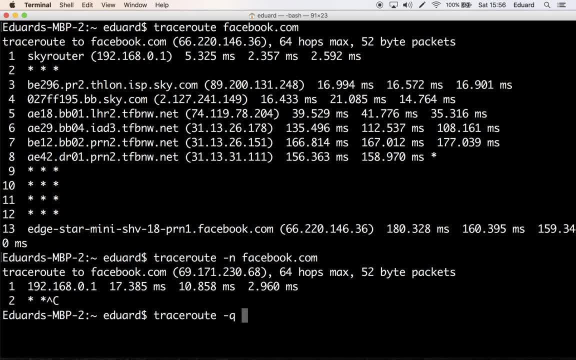 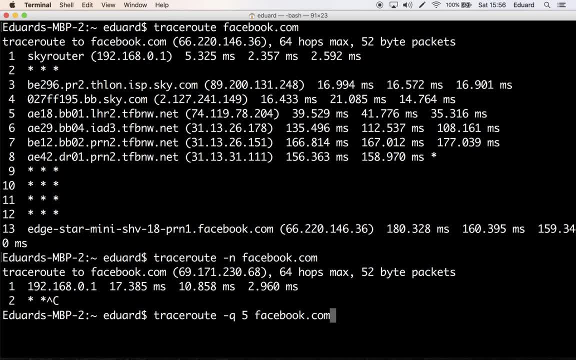 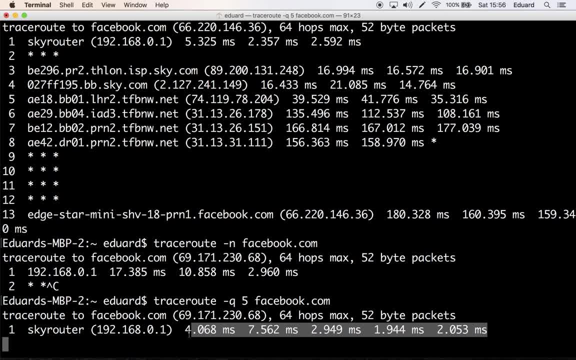 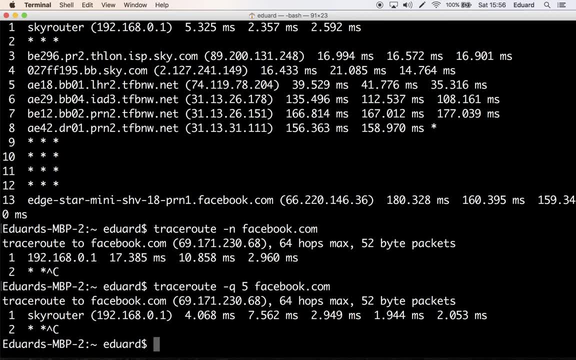 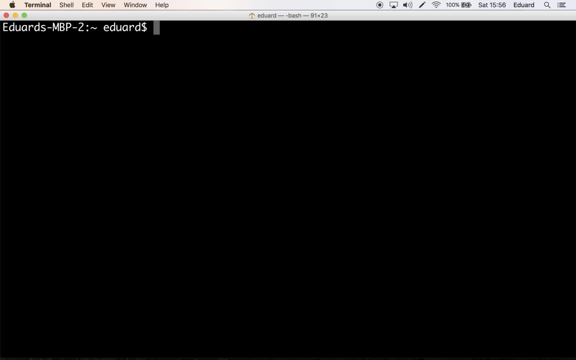 And as you can see here already in my first line, it has shown five RTT values from my skyrouter. Let me cancel the command, Let me clear the screen. Another interesting option would be to pre-set your TTL value. By default, TTL value is set as 1.. 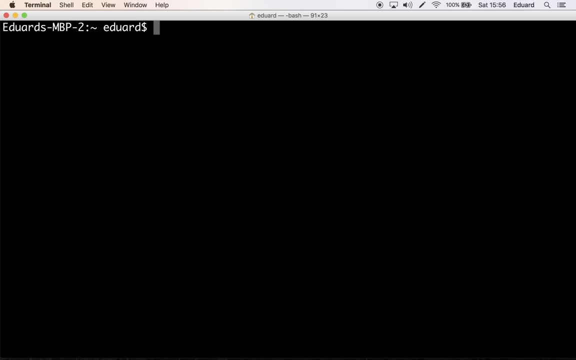 which states that it will begin with the first router in the route. you can change that by using the minus f option and let's say 10.. so using the the minus f or dash f option. um, this takes an integer as an argument and this argument is the new value of ttl. so this would be the initial ttl value that your traceroute command. 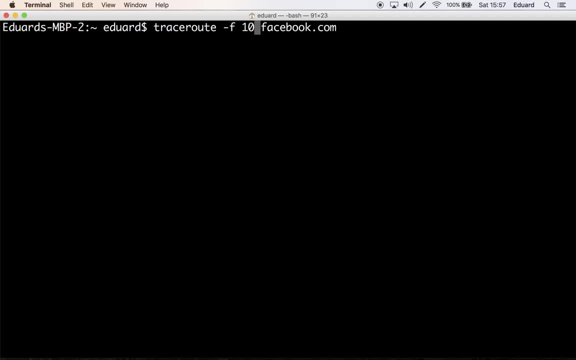 will start with right, so i hope you have grasped quite easily what i've shown you in this video. that's it for today. i hope you found the tutorial useful. go ahead and play with traceroute to learn more. don't forget to subscribe and i'll see you in the next video.